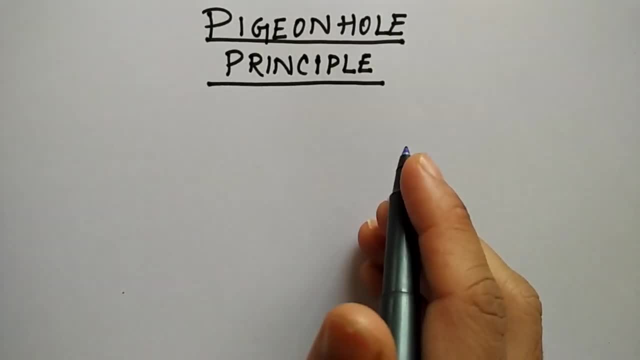 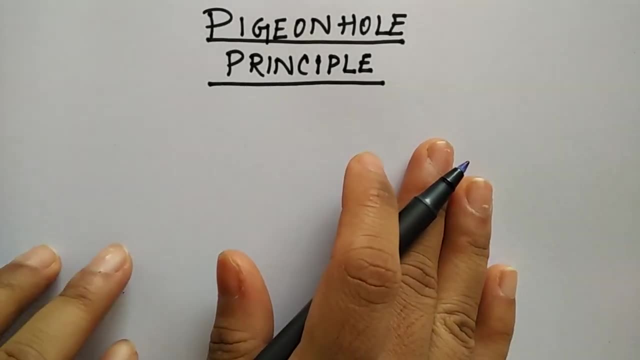 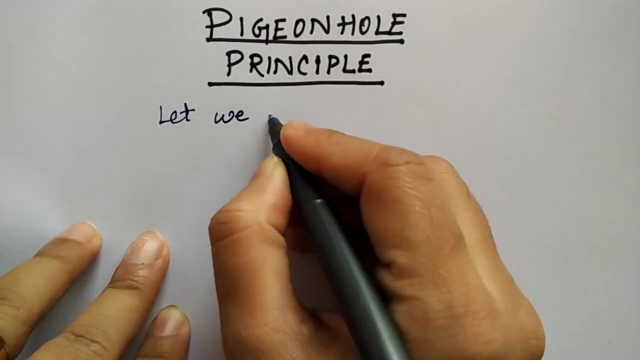 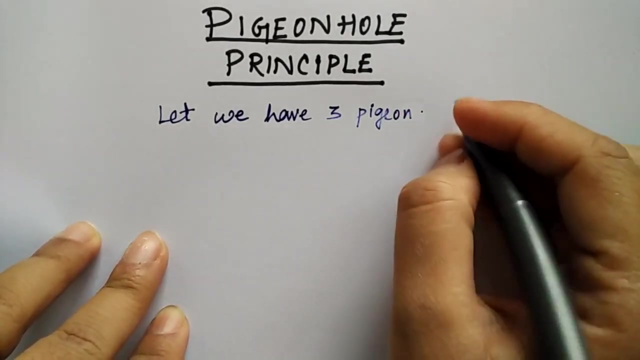 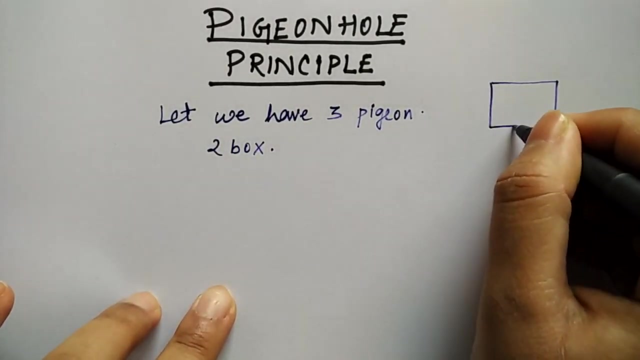 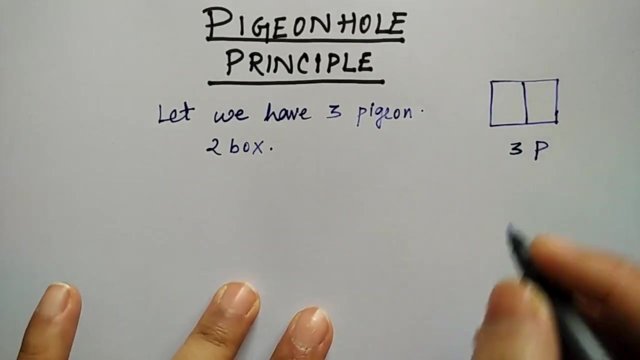 Hello student. today's topic is Pigeonhole Principle. Let me explain to you first why it is called as Pigeonhole Principle. Let's say we have three pigeons, We have three pigeons and we have two boxes. It means I have a container in which I am having two places, But I have how many pigeons? Three pigeons. 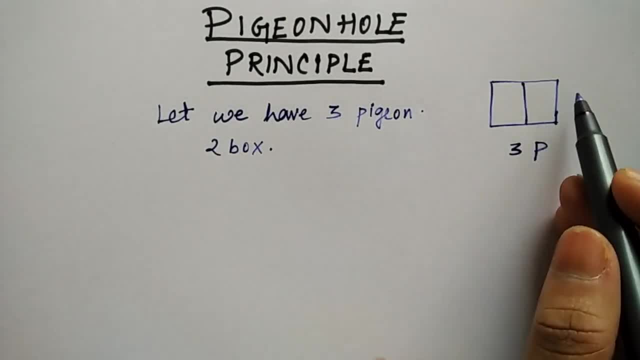 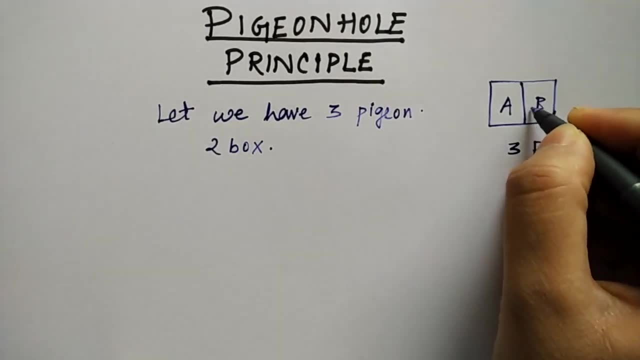 So how to accommodate three pigeons into two boxes. So there are three pigeons: A, B, C. I will keep pigeon A here and pigeon B here. So where the pigeon C will go, Either we have to keep that C one with A or we have to keep it with B. 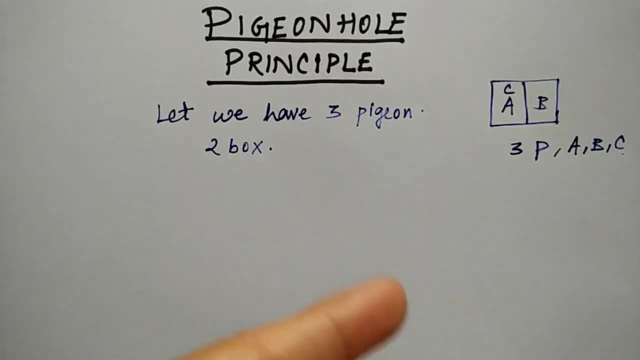 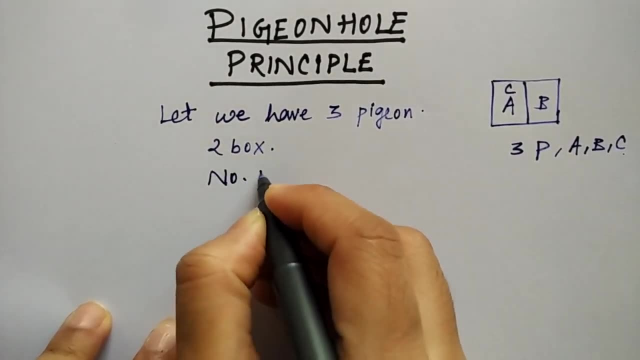 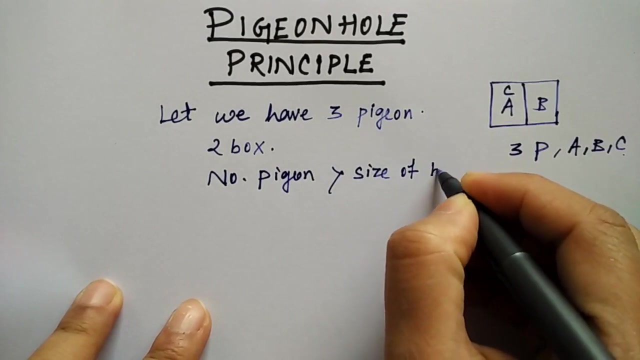 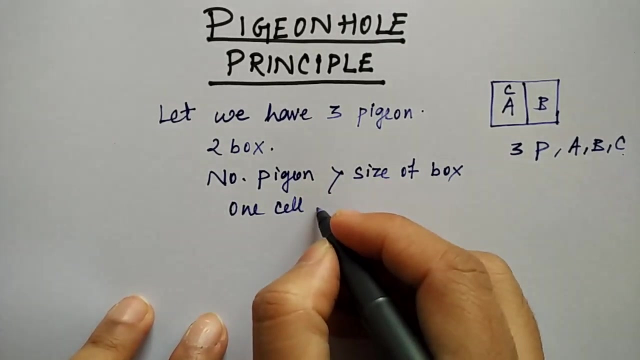 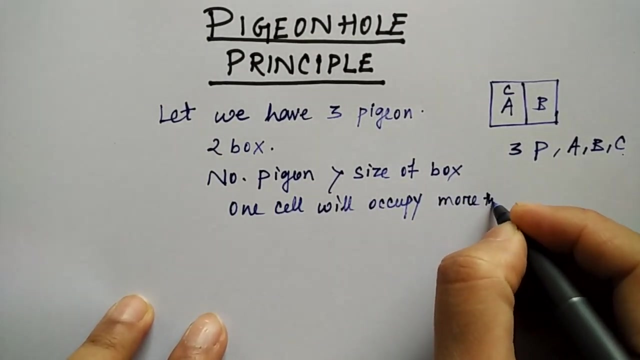 So any of the two places is occupying two pigeons and the other one is occupying one pigeon. So this is the concept of pigeonhole: When the number of pigeons is more than the size of the box, then one cell will occupy more than one pigeon. 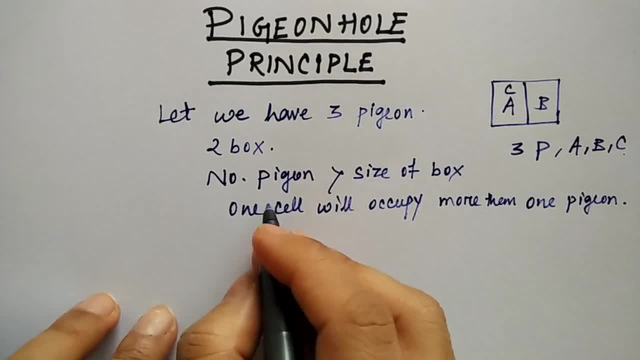 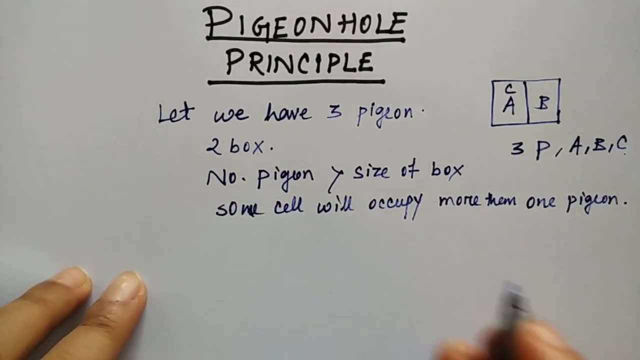 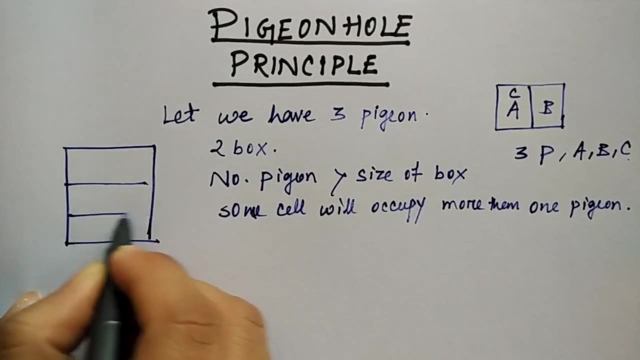 Not one cell, We can tell it as some cell. Okay, Because if Let's say another example, we will see. I have the box, Six places. I have This is the box And I have got some ten pigeons. How to keep the ten pigeons Here? 1, 2, 3, 4 and 5, 6.. 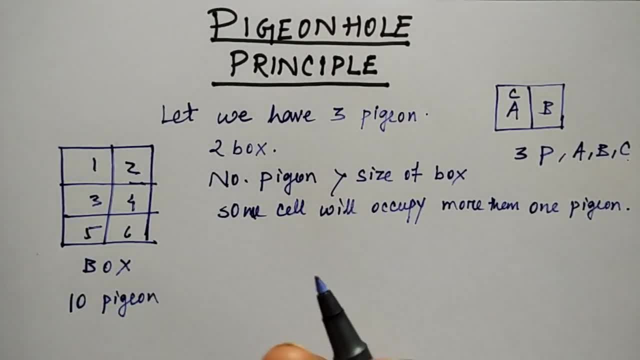 Where the other pigeons will go. We have to accommodate them somewhere right. The other four we can keep it here, here, here, here. So this: These four places are having two, two pigeons and these two are having single pigeons. 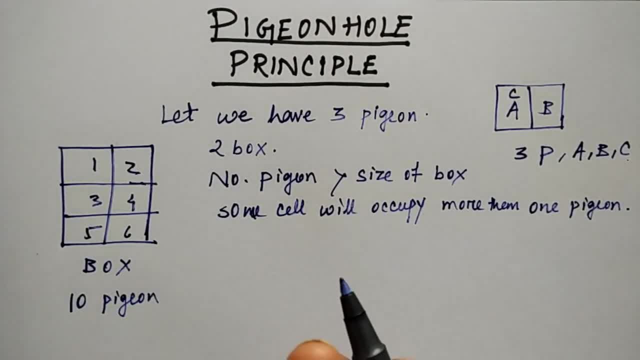 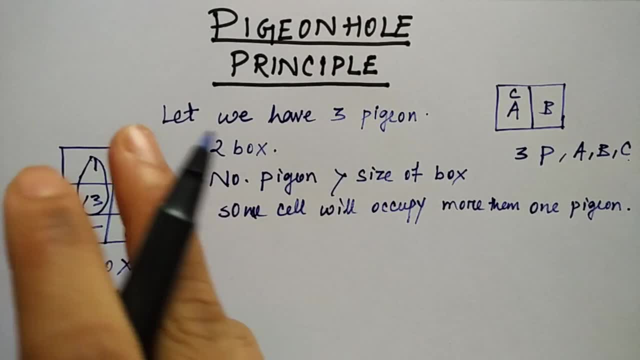 Where the other pigeons will go. We have to accommodate them somewhere, right? The other four we can keep it here, here, here, here. So this four places, Okay, This are having two, two pigeons, and these two are having single pigeons. 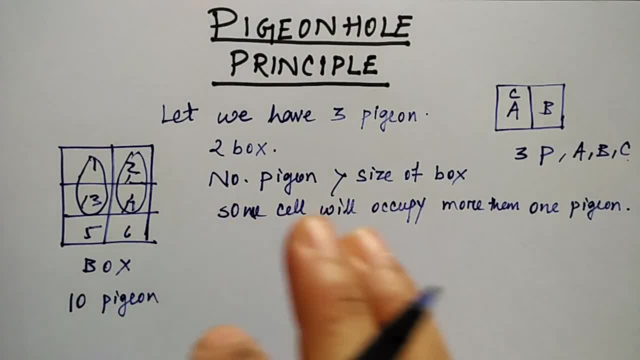 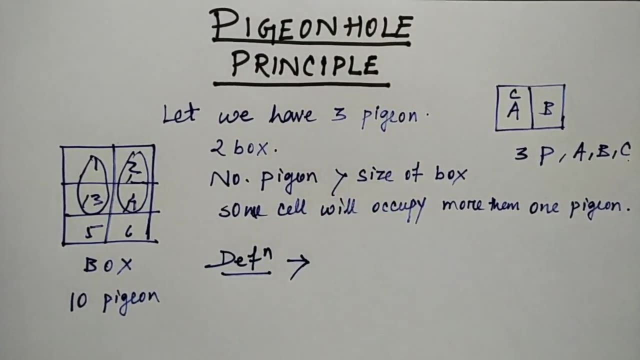 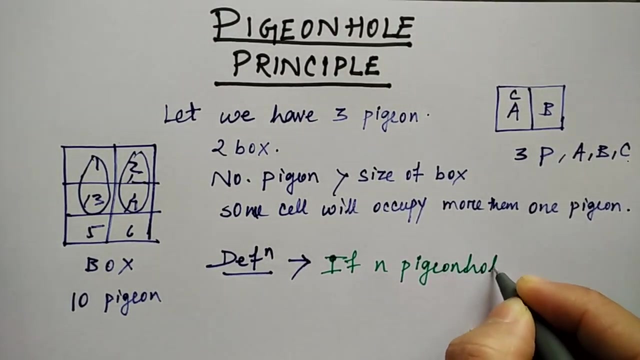 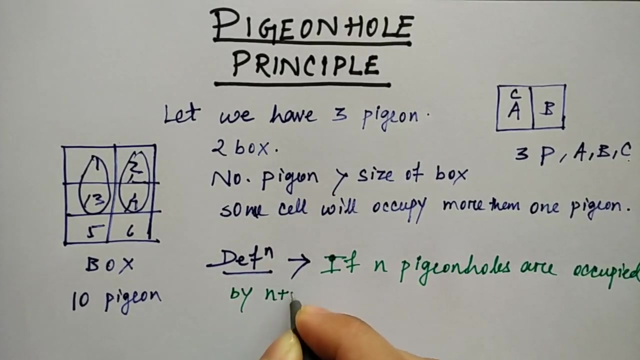 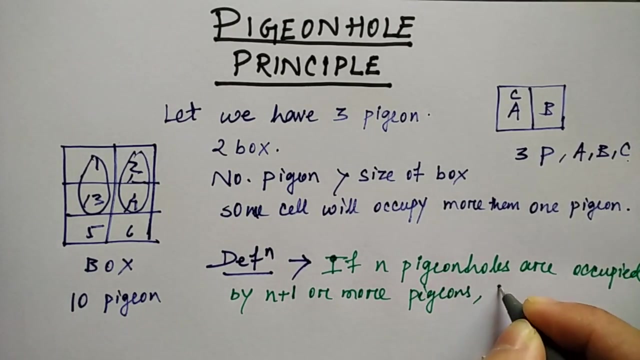 So this is how, like how can you accommodate the pigeon into the pigeonhole when the number of pigeons are more than the number of holes? That is the concept. So the definition we'll see. Definition is: If n pigeon holes are occupied by n plus one or more pigeons, then at least one pigeon occupy. 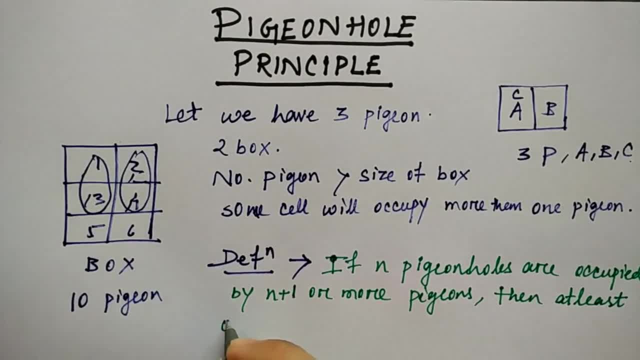 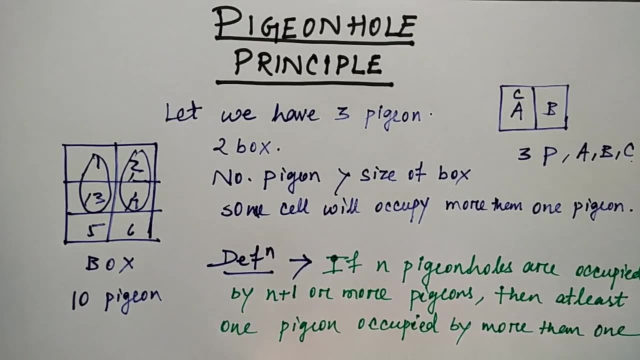 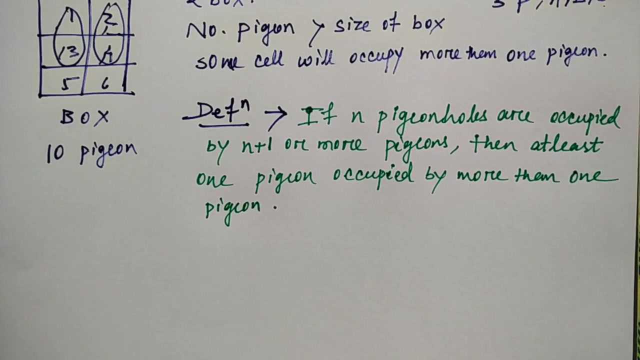 If n pigeon holes are occupied by n plus one or more pigeons, then at least one pigeon occupy, or at least one pigeon occupied by more than one pigeon If n pigeon are occupied by n plus one. If n pigeon are occupied by n plus one or more. 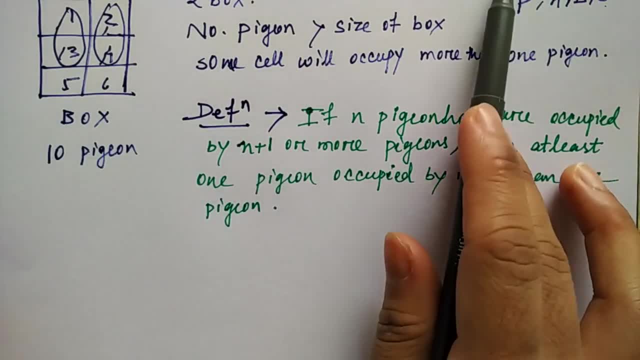 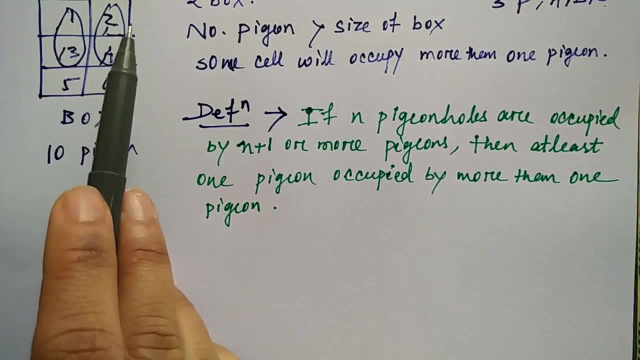 If n pigeon holes- let's say two pigeons here, let's say six pigeon holes are there- are occupied by n plus one. Yes, It is. obviously the number is more than 1 pigeon. Okay, Right of pigeons are more than the number of box size or holes in the box. then at 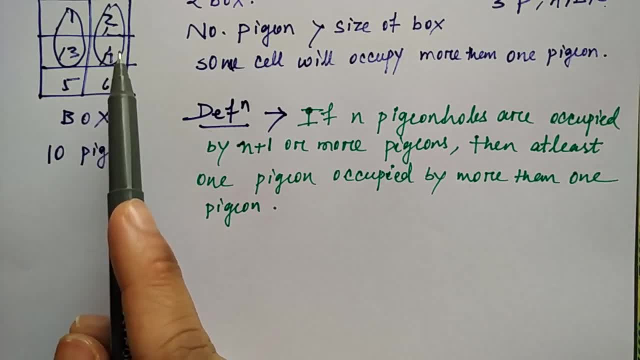 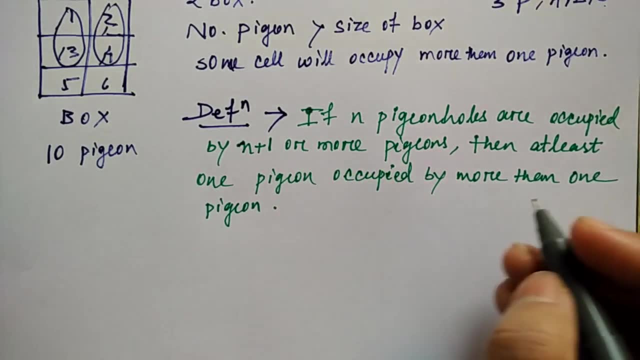 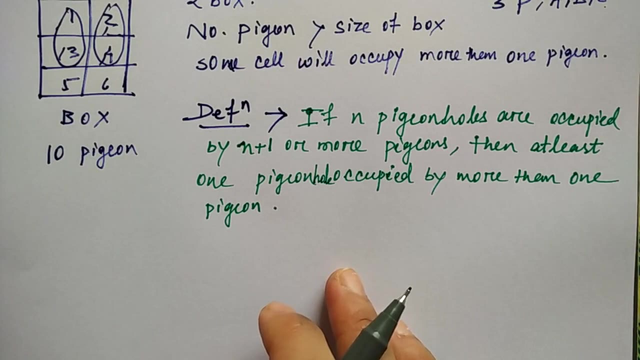 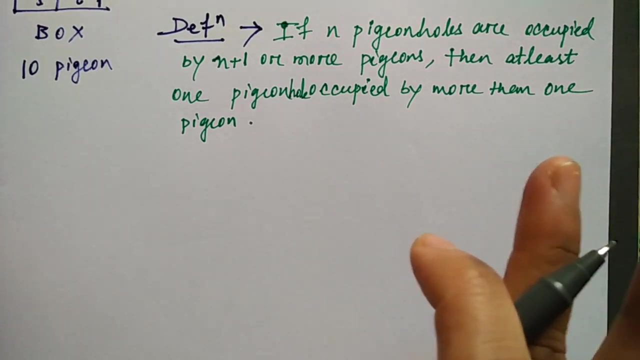 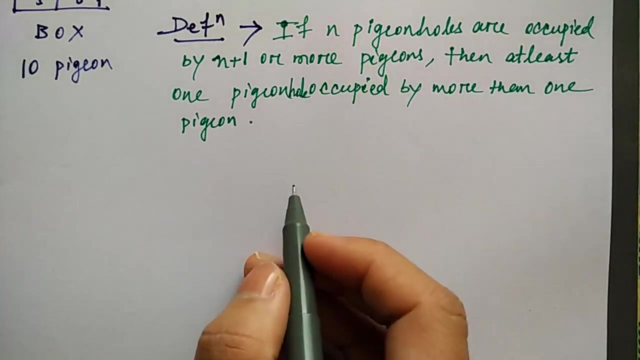 least one pigeon occupied by more than one pigeon hole. sorry, this is a pigeon hole. so let me make it more clear. according to the definition it is, if n pigeon holes are occupied by n plus 1 or more pigeon, then at least one pigeon hole occupied more than one pigeon, so let's say n pigeon whole- means we have 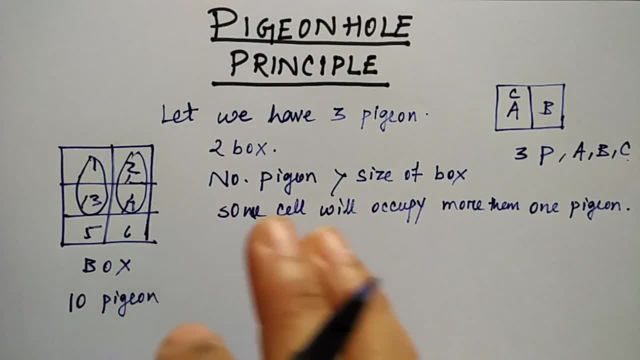 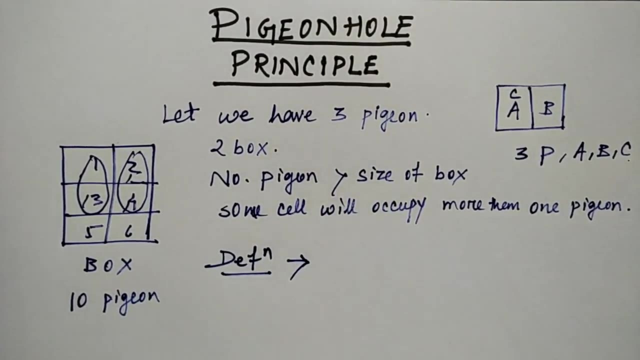 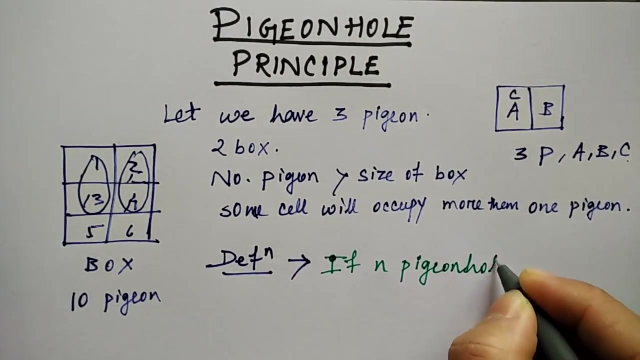 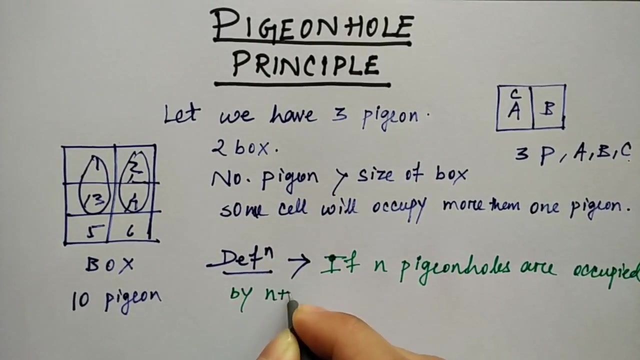 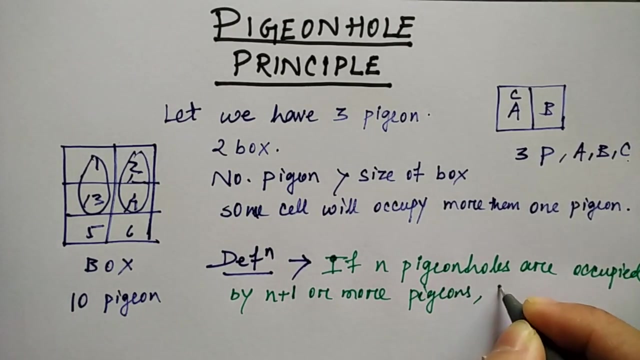 So this is how, Like how, can you accommodate the pigeon into the pigeonhole when the number of pigeons are more than the number of holes? That is the concept. So the definition we will see. Definition is Then: if N pigeon holes are occupied by N-plus-one or more pigeons, then at 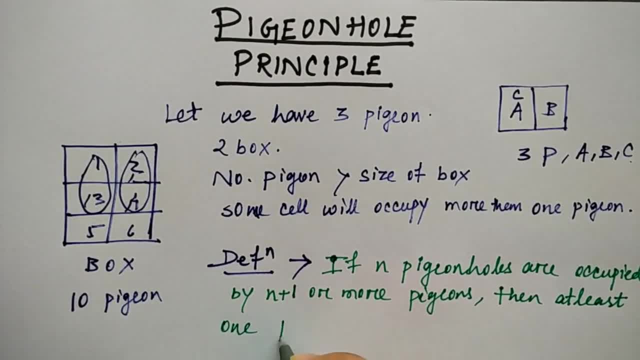 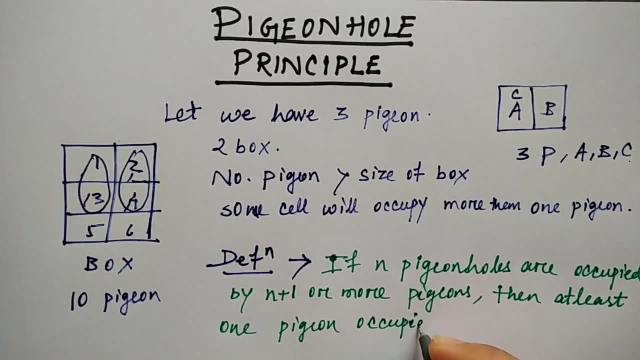 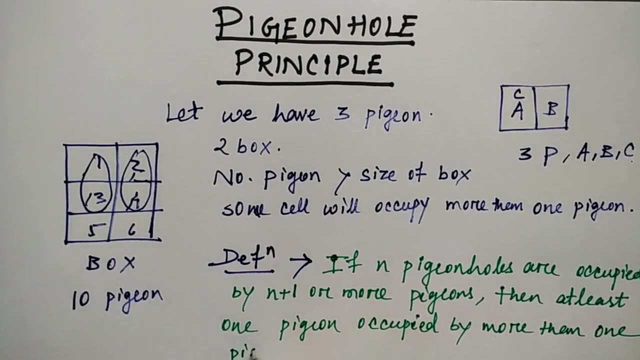 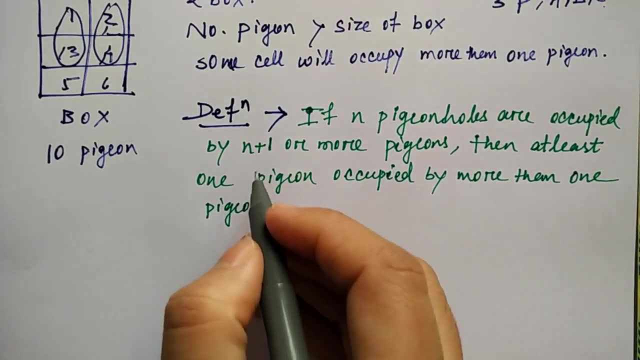 least one pigeon occupies. If N piggy hull are occupied by N-plus-one or more, Then if n pigeon holes are occupied by N-plus-one or more occupy, or at least one pigeon occupied by more than one pigeon. so this is the definition if n pigeons are occupied by n plus one or more pigeon. if n pigeon. 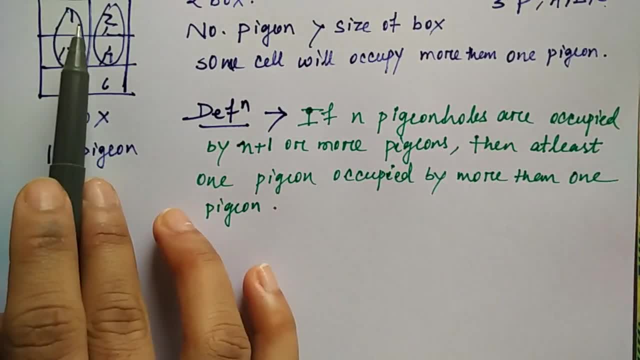 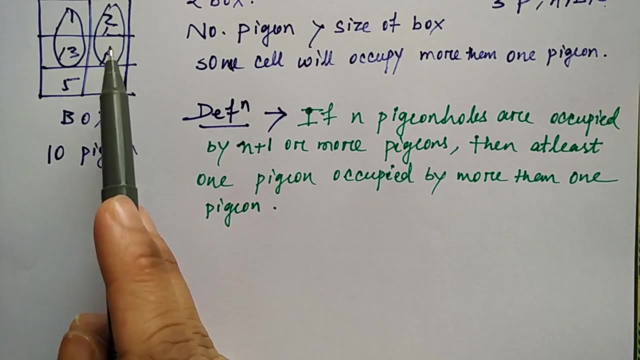 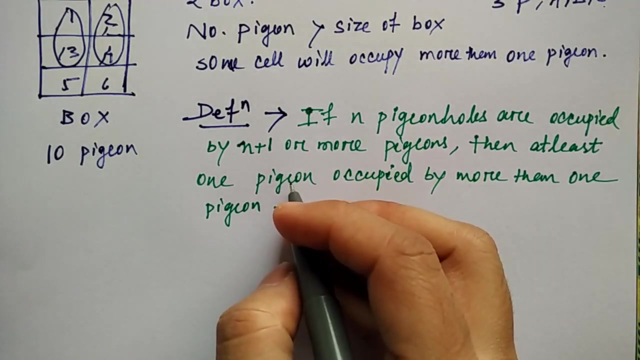 hole, let's say two pigeon here, let's say six pigeon hole. pigeon holes are there, are occupied by n plus one. yes, it is obviously the number of pigeons are more than the number of box size of holes in the box. then at least one pigeon occupied by more than one pigeon hole. 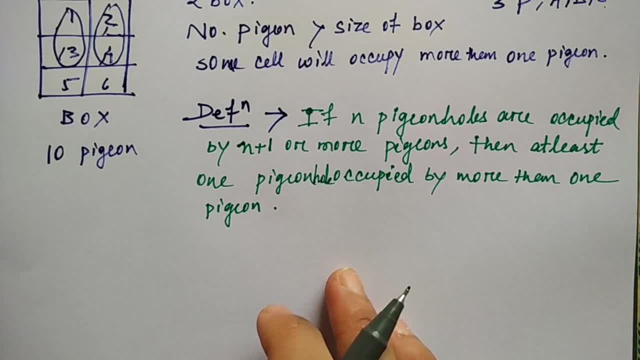 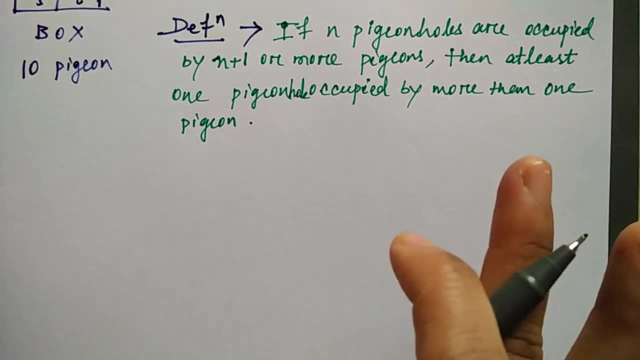 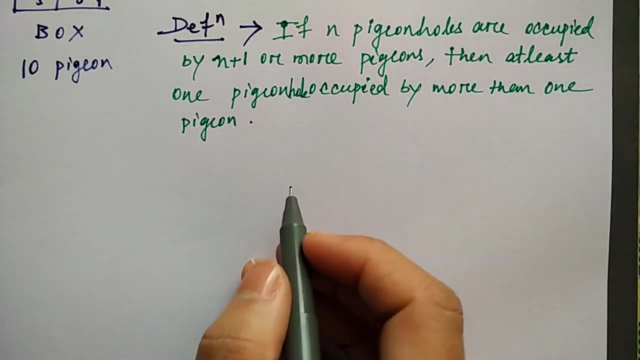 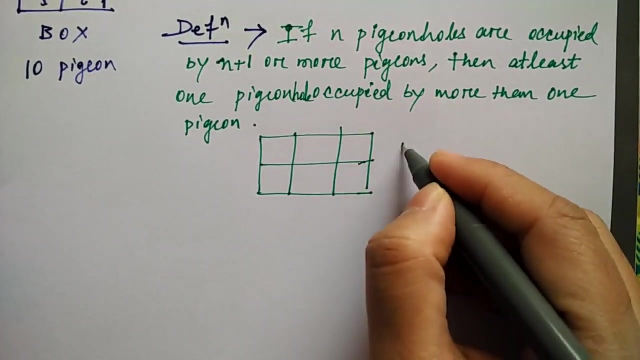 sorry, this is a pigeon hole. so let me make it more clear. according to the definition it is: if n pigeon holes are occupied by n plus one or more pigeon, then at least one pigeon hole occupied more than one pigeon. so let's say n pigeon hole means we have got here six pigeon hole. pigeon hole are: 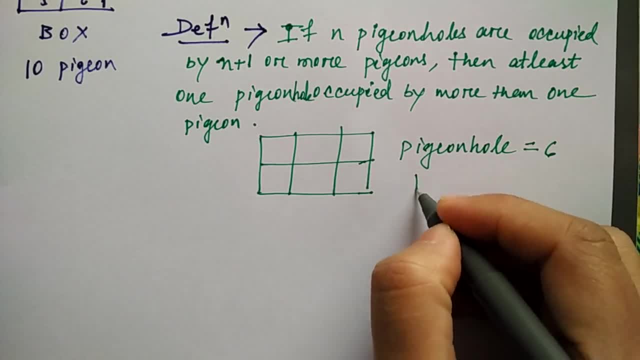 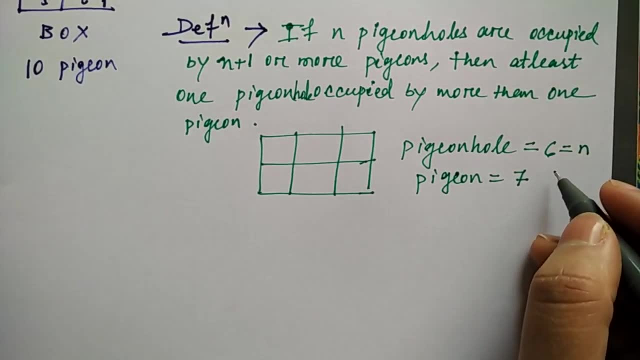 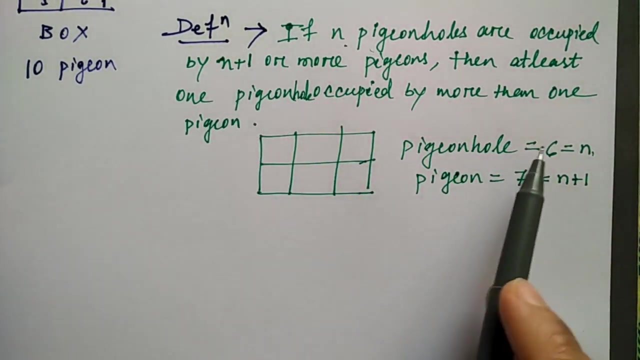 six, and let's say I have number of pigeon equal to seven. so here, if pigeon is n, or sorry, if pigeon hole is n, the number of pigeon is n plus one. so if n pigeon hole are occupied by n plus, if all this pigeon hole should occupy all this pigeon, 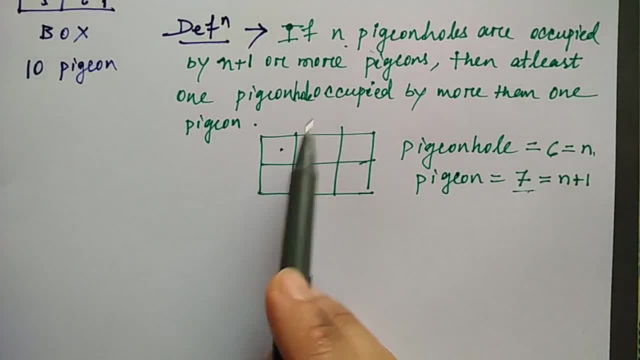 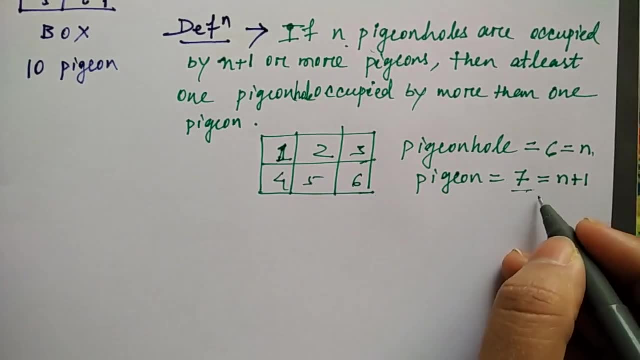 that is one more than the pigeon hole, then at least one pigeon hole occupied by more than one pigeon. that is obviously correct, because if you are keeping one, two, three, four, five, six, where the seventh one will go, you have to keep it with some other pigeon, right? so it is saying that at least.